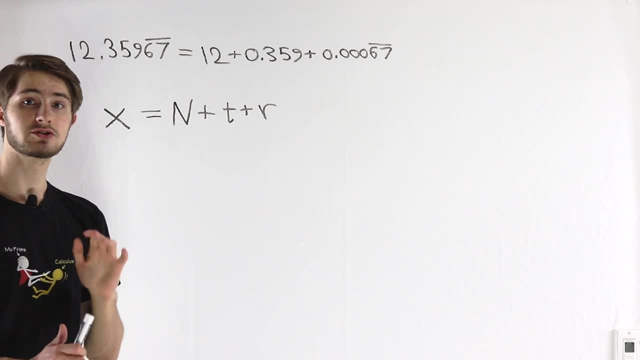 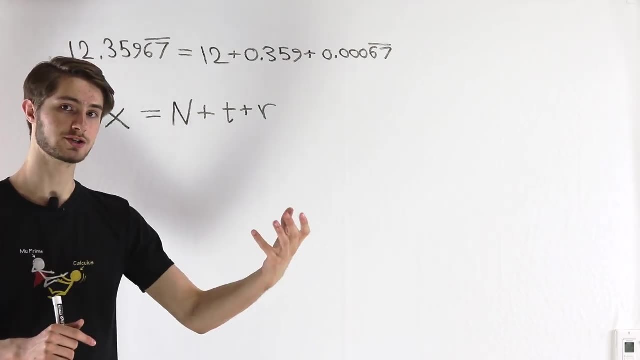 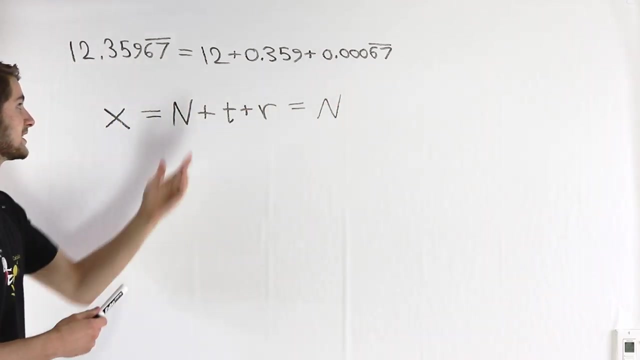 that each of these three terms is a rational number, because the rational numbers are closed under addition, which means one rational number plus another rational number must give us a rational result. In this case, we already know that n must be a rational number because it's an integer. In this case, 12 is just 12 over 1.. Every integer is a rational number. Now, when we take a 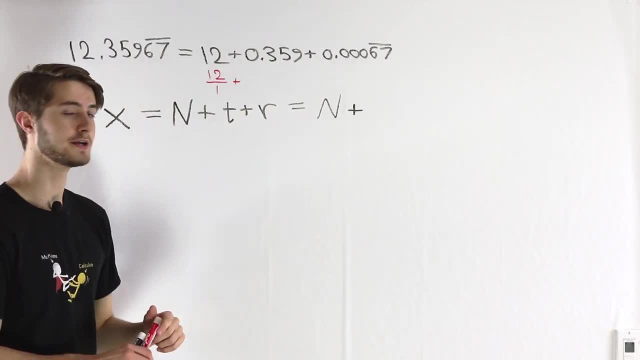 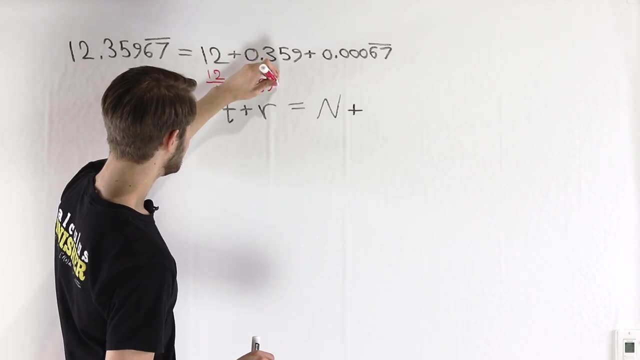 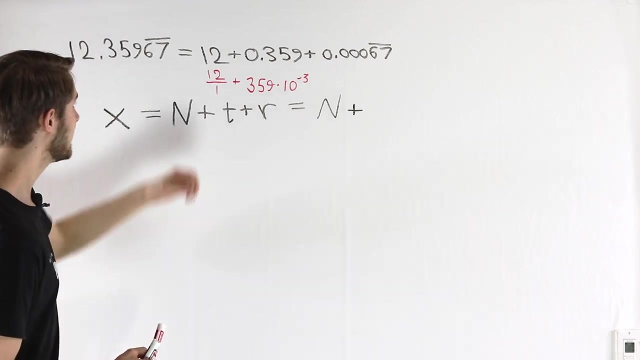 look at this terminating decimal part: 0.359. notice that we can write 0.359 as 359 times 10 to the negative 3.. If we multiply by 10 to the negative 3, that has the effect of taking our number 359 and. 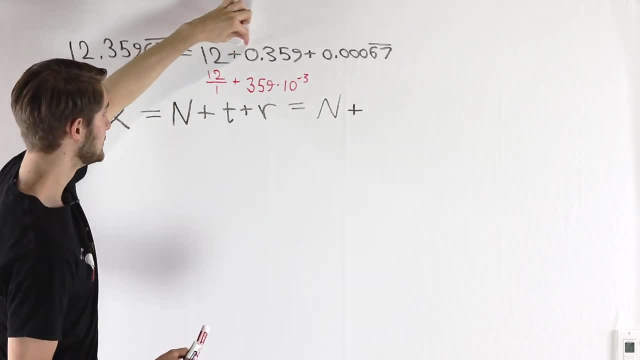 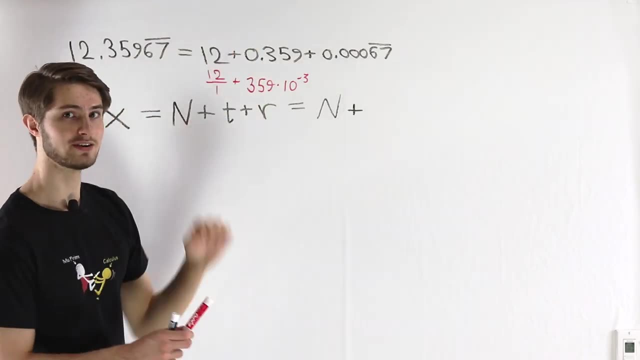 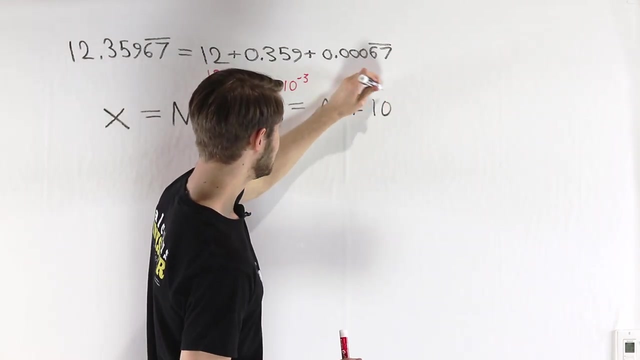 shifting the decimal place over three times, so we get 0.359 as the result. Each of these is a rational number and therefore if we do that, we get a rational number. 0.359 must be rational as well For a general terminating decimal. we can write that as 10 to. 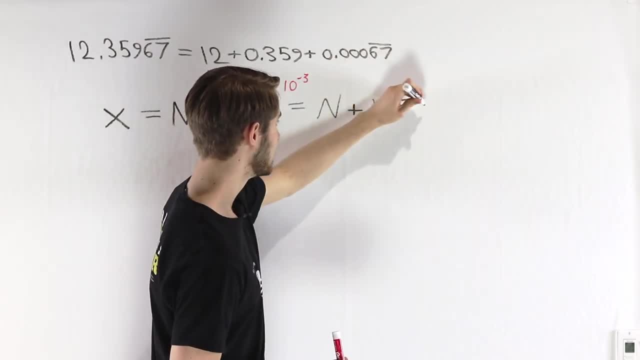 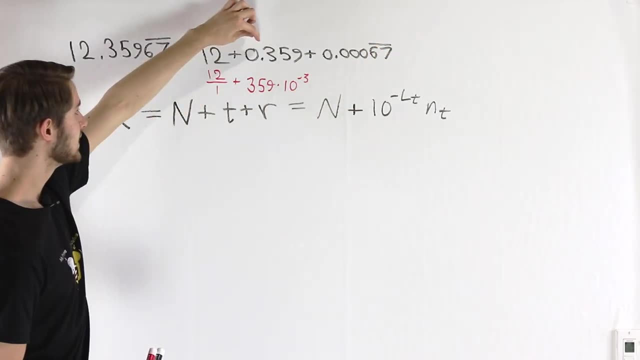 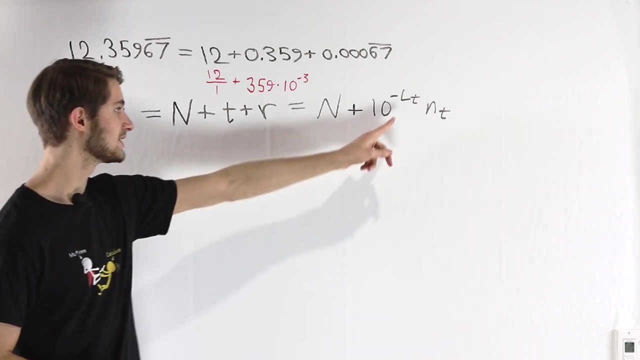 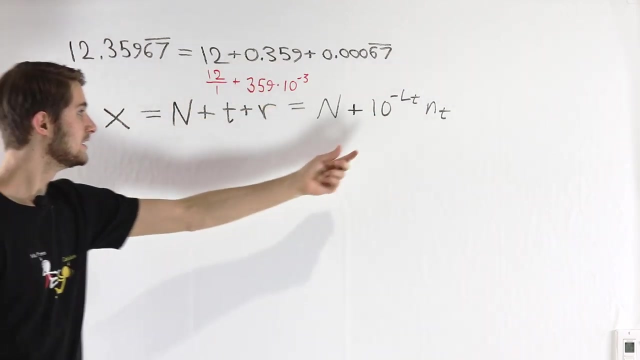 the negative LT times NT. In this case, LT is the length of our terminating decimal. The length of 359 was 3 because we had three digits. So for a general terminating decimal, T it'll have a length. LT And NT is just the digits in that decimal, In this case 0.359,, NT was 359.. Now, finally, we have 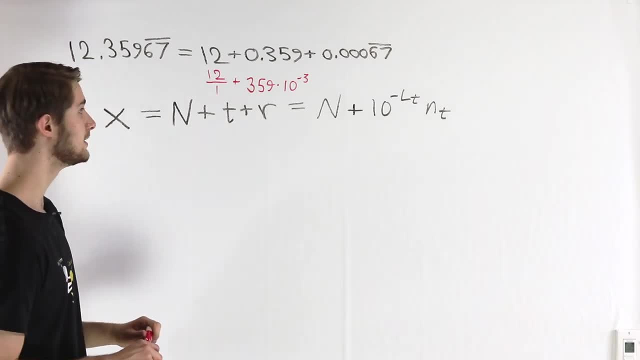 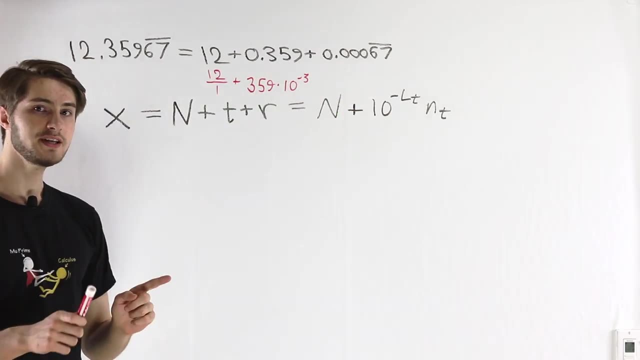 to look at the repeating part, and that's going to be the most difficult. But now that we've isolated it by itself, we're going to have a little easier time dealing with it. For the repeating decimal, let's try the same trick that we did with the terminating decimal, namely that we want to write. 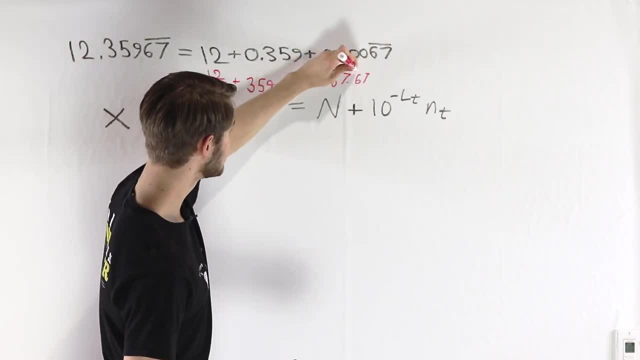 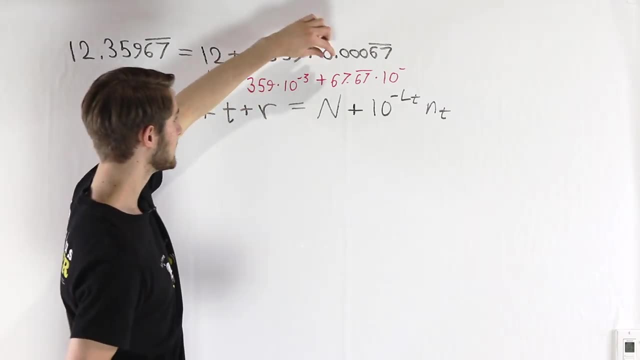 this as 7 to the negative LT. So we're going to write this as 7 to the negative LT And we're going to have 67.67 repeating times, 10 to the negative of some value In this case, if we want to get from. 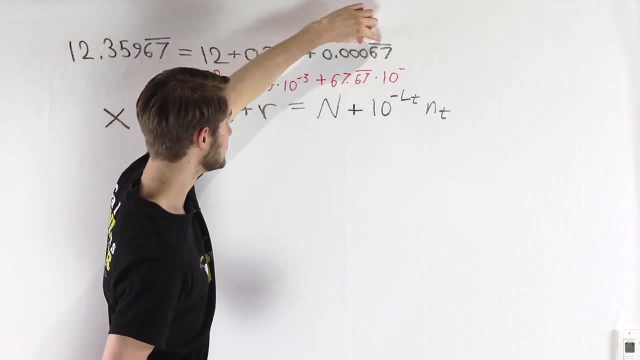 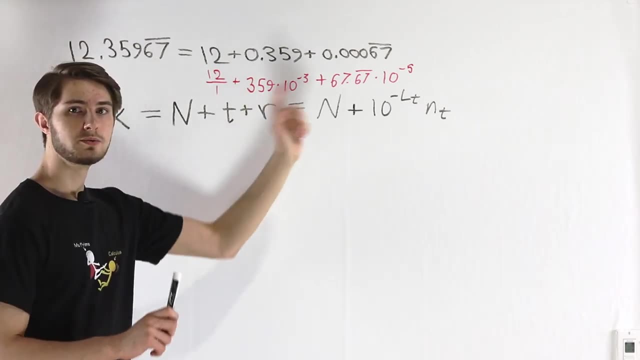 67, all the way over to 1,, 2,, 3,, 4, 5 places down. we need to multiply by 10 to the negative 5.. So we know that for our repeating decimal in general, we're going to need to multiply by 10. 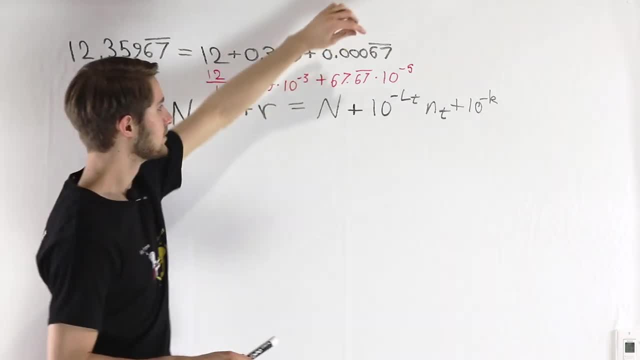 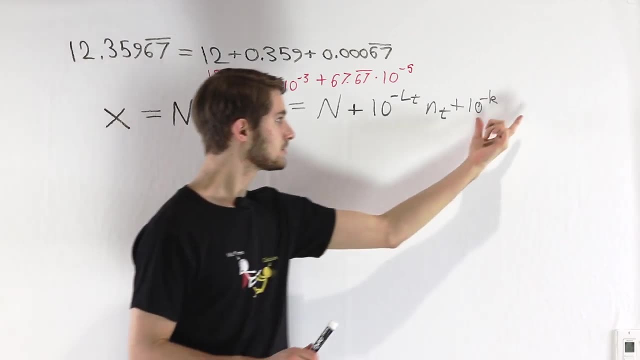 to the negative something. We'll just call it k, so that we shift the number over until it starts to the left of the decimal place From here. we want to multiply this by something For the terminating decimal. that something that we multiplied was just those. 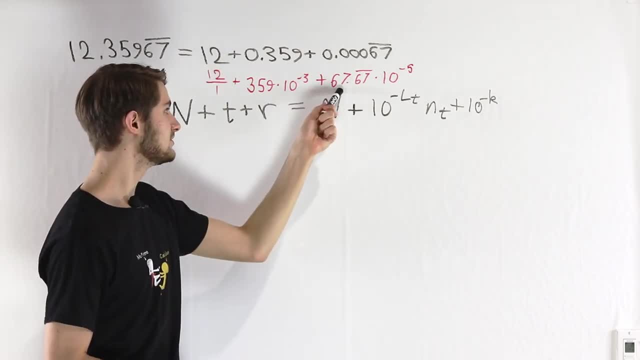 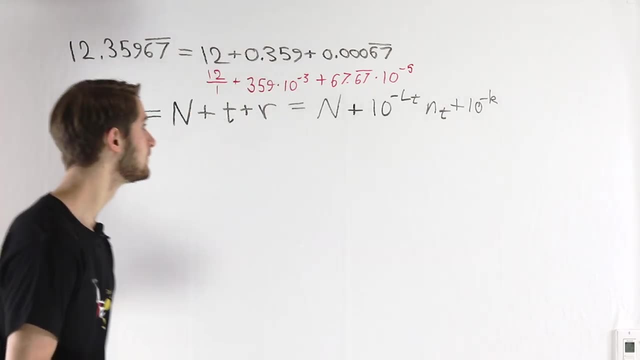 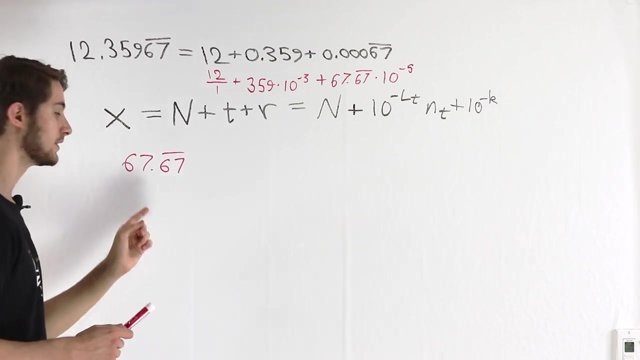 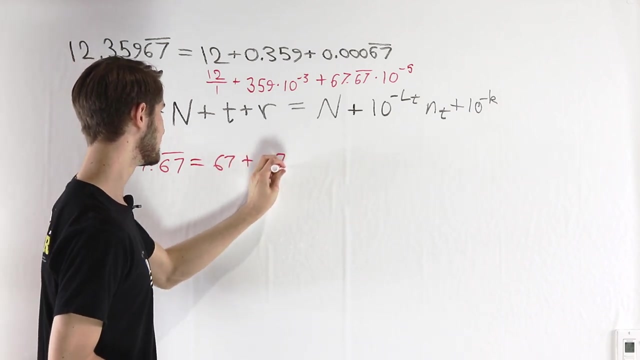 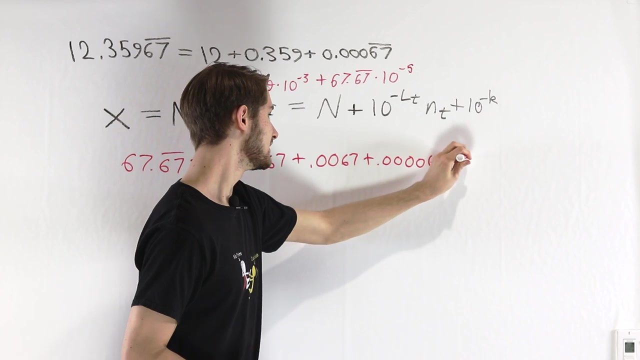 digits 359.. But in this case we still have an infinite number of decimal places, So we need to do a little more work to figure out what goes here. Let's think about what is 67.67 repeating. One way that we can express this is as 67 plus 0.67 plus 0.0067 plus 0.000067, and so on. 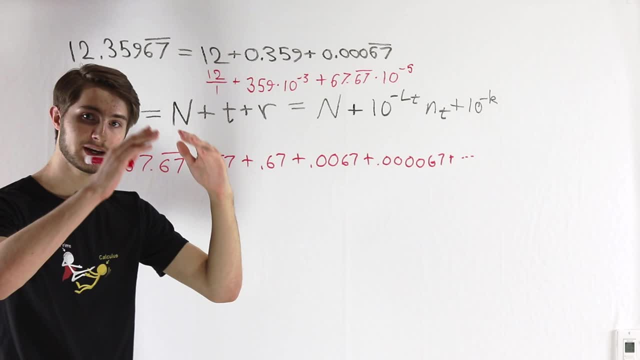 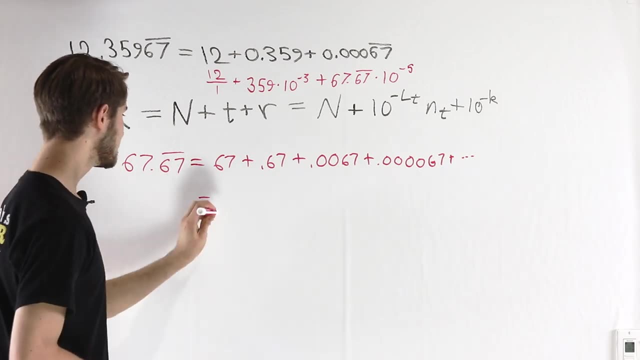 If we can write this with sigma notation so that we get one nice sum, then we can do some calculations on it to figure out what exactly it equals. So let's see if we can write this in a nice compact form. First of all, 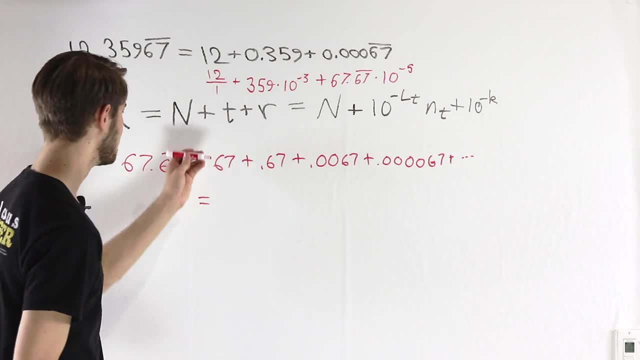 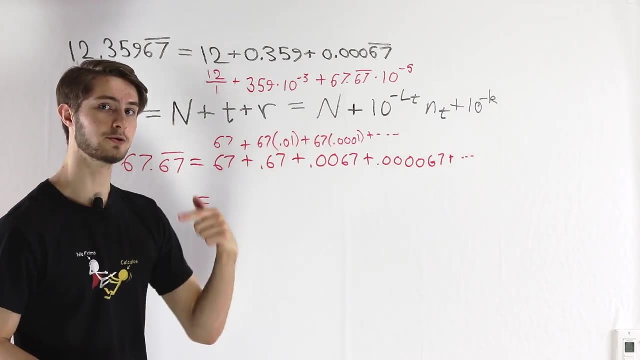 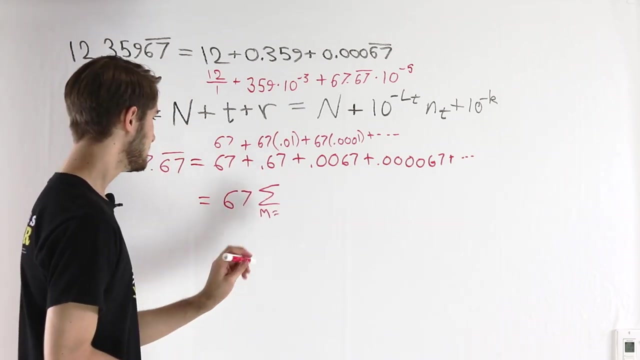 we know that we could factor out a 67 from each of these terms. So in each case we're factoring out the 67 and we're left with some power of 10.. So we can write this as: 67 times the sum from, let's say, m equals 0 to infinity of what are we adding up in each of. 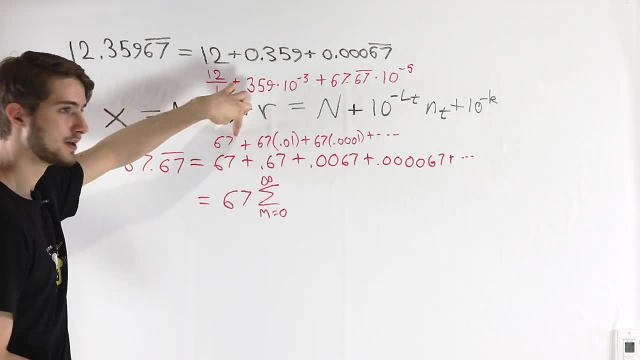 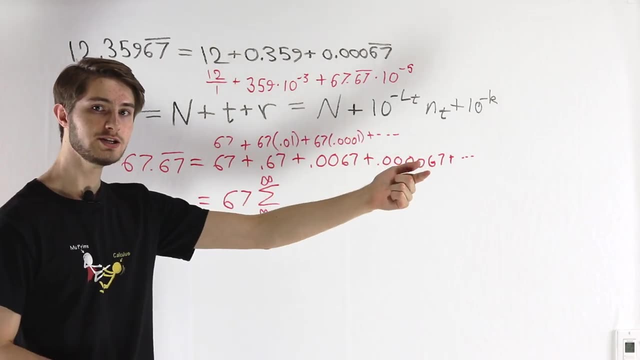 these terms? Well, first we had 1, and then we had 0.01.. And then we had 0.0001.. How are we getting from each term to the next? Well, we know that 1 is 10 to the 0.. 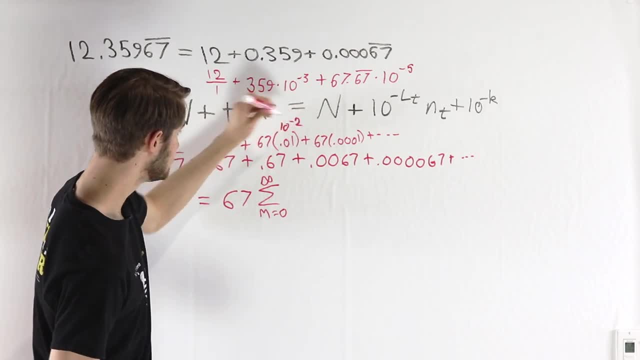 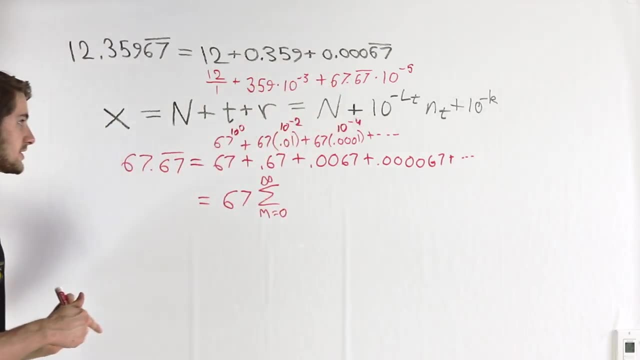 0.01, that's 10 to the negative 2.. 0.0001, that's 10 to the negative 4.. So each time we go from one term to the next, we're going to multiply by 10 to the negative 2.. And that makes sense, because multiplying 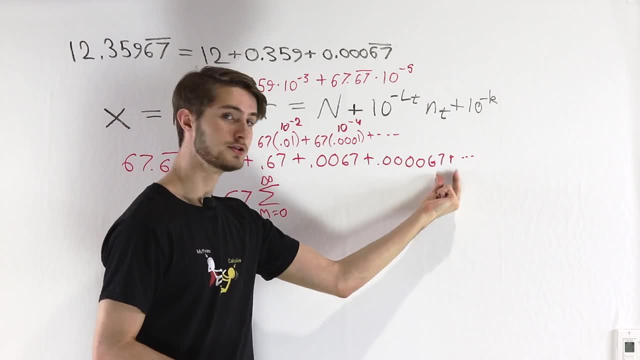 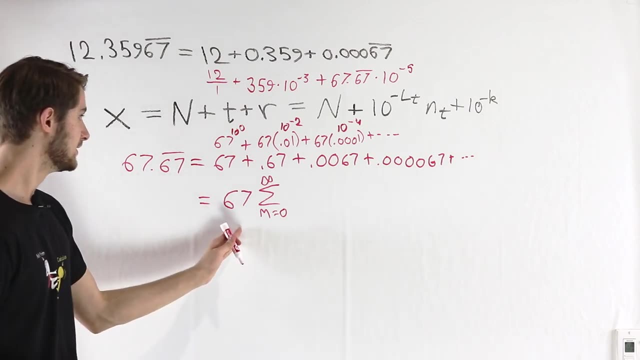 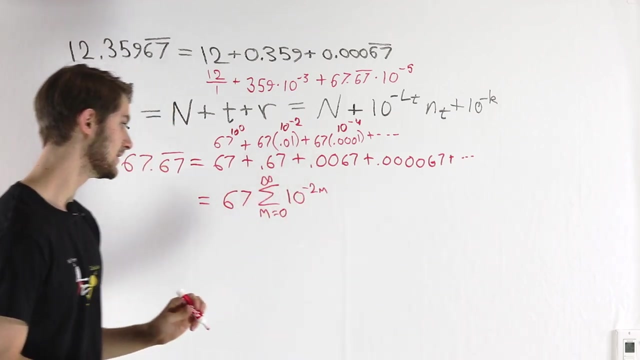 by 10 to the negative 2 means we shift the decimal two places over, So we get our repeating decimal expansion. Therefore, our sum is going to be: from m equals 0 to infinity, of 10 to the negative 2 times m, or equivalently, 10 to the negative 2 to the power of m. This 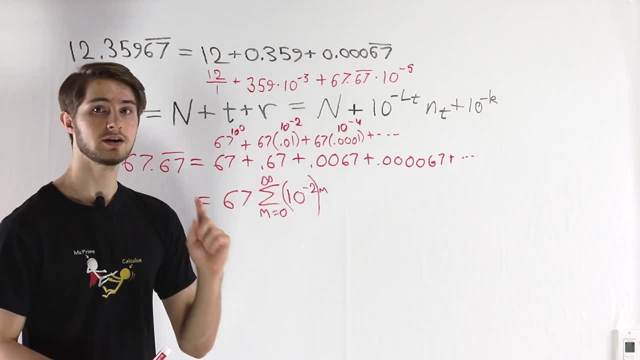 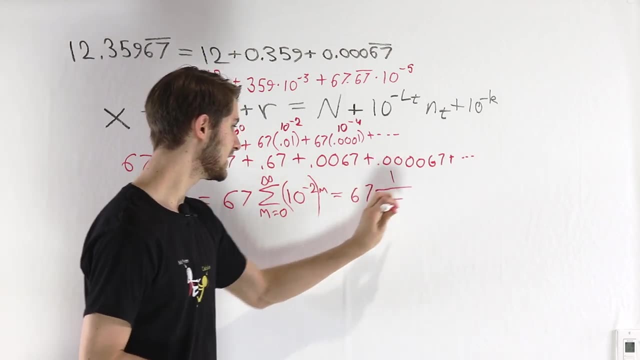 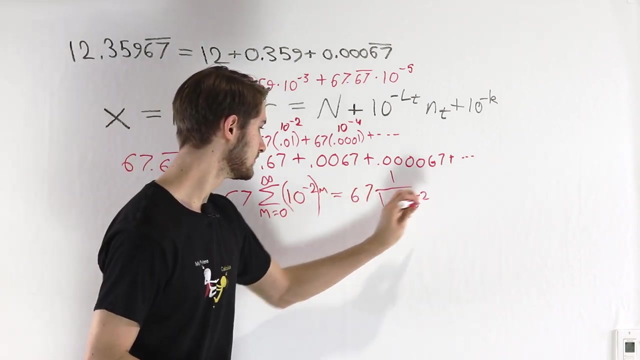 is an infinite geometric series, which means that we can evaluate it with the methods that we know. This geometric series must equal 1 over 1 minus the common ratio r, And in this case the common ratio is 10 to the negative 2.. 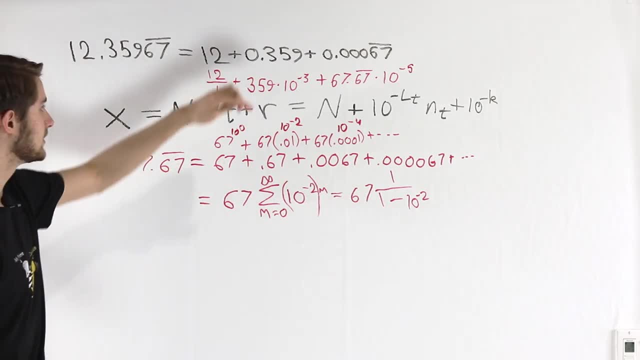 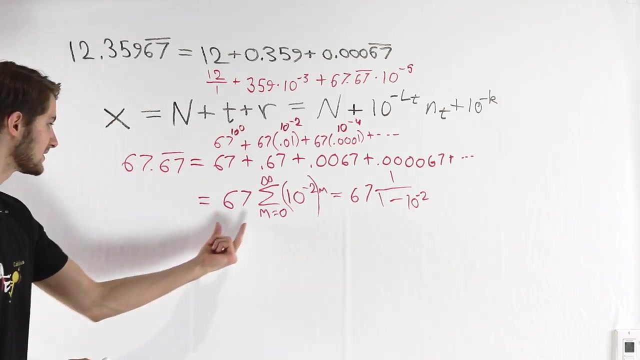 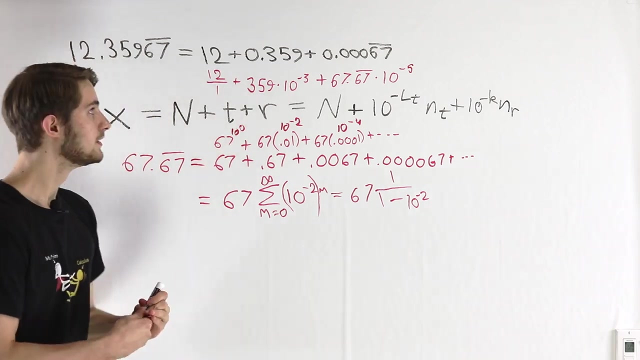 So that's what our repeating decimal expansion looks like for 0.00067 repeating. How can we take this and write it for an arbitrary repeating decimal? All we have to do to answer that question is take all of the cases with 67 and replace it with the arbitrary number n, sub, r, the 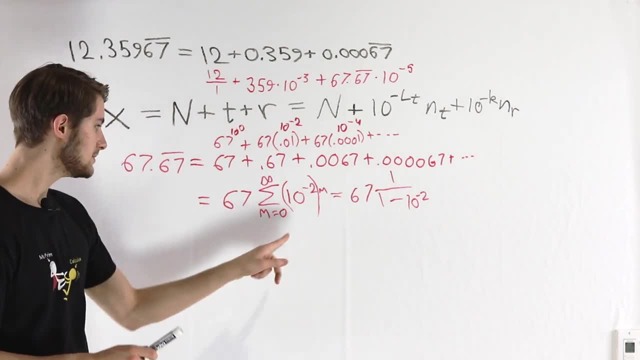 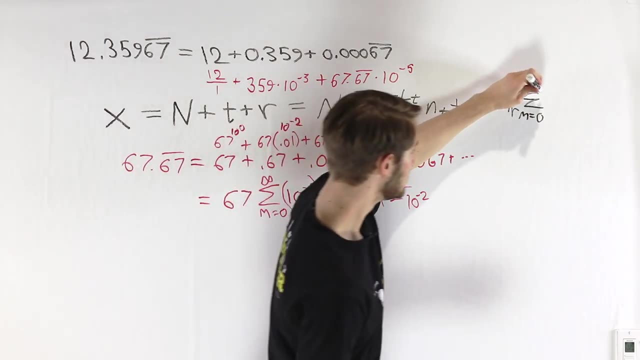 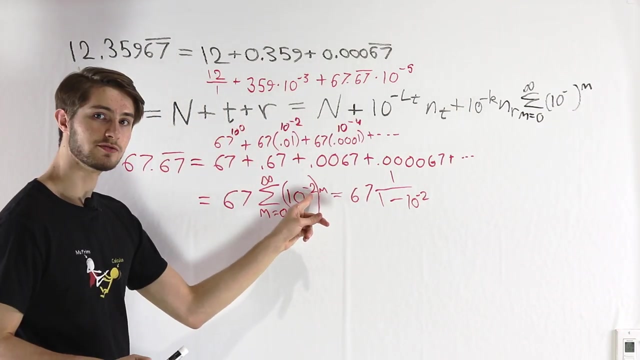 digits of the repeating decimal And then, if we keep writing out what we have here, we'll have the sum from m equals 0 to infinity, of 10 to the negative something to the power of m. Remember that 10 to the negative 2, we chose the number 2 there because the line 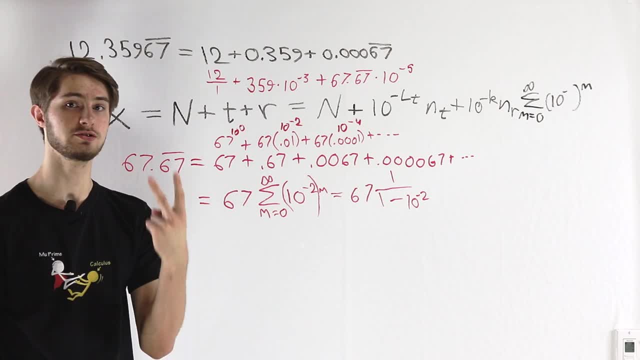 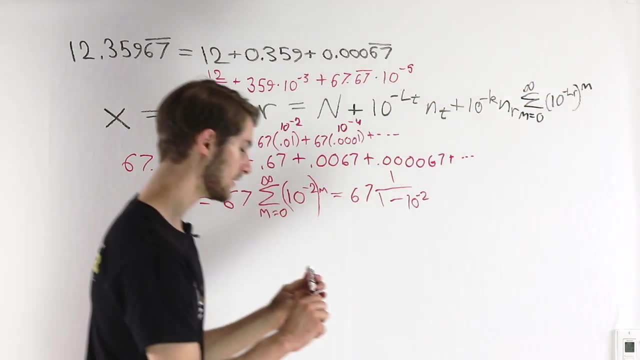 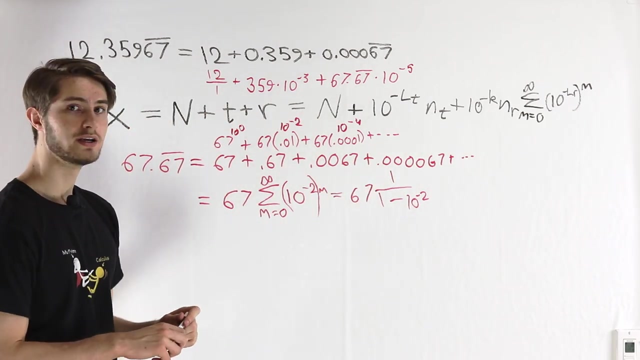 is 0. So the length of 67 is 2,. 67 has 2 digits. For an arbitrary repeating decimal it's going to have some length- l sub r- And every time we add another instance of that repeating sequence it's going to be shifted over. l sub r places to the right. So we multiply. 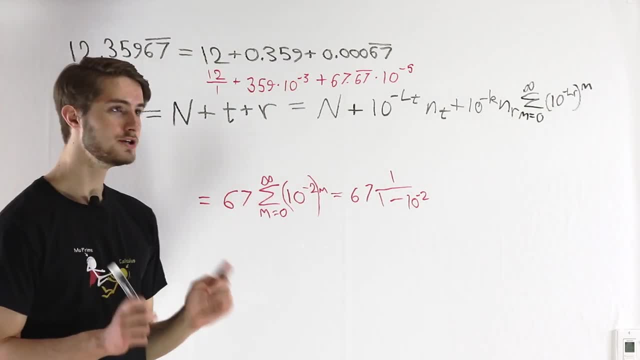 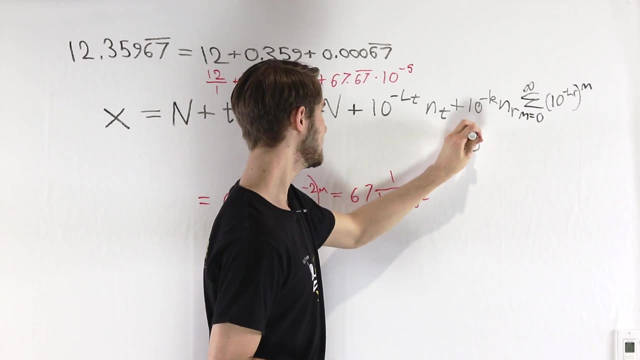 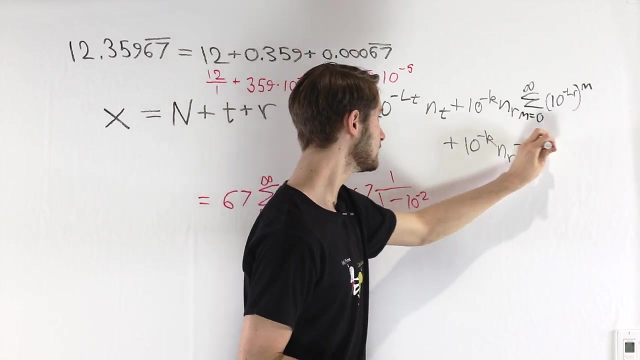 by 10 to the negative l sub r. And, just like before, at the end here we have a geometric series and therefore we can evaluate this as 10 to the negative k times our repeating decimal digits: n sub r times 1 over 1, minus that common ratio, 10 to the negative l sub. 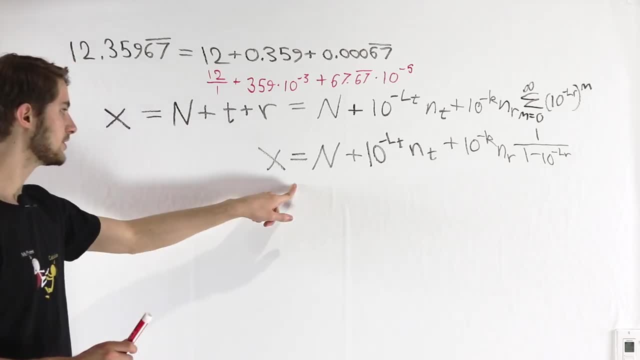 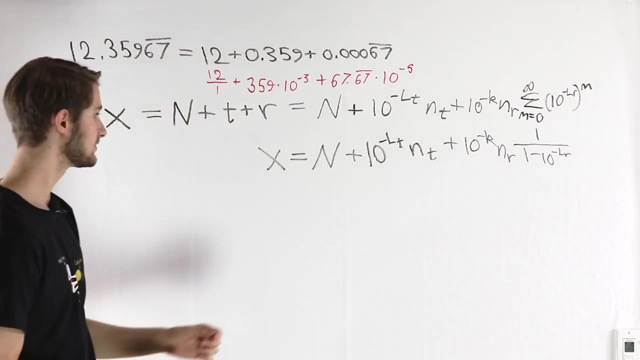 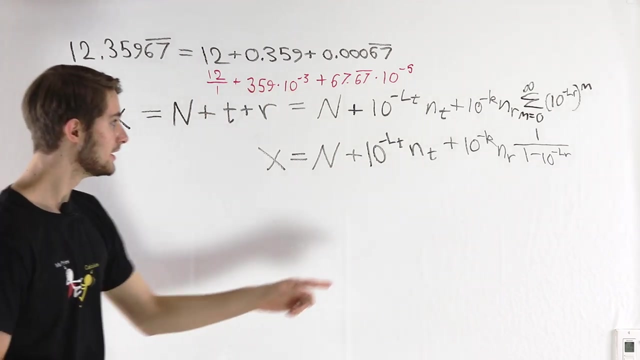 r. So this is one way we can express our number. with a repeating decimal x. We can add up first the original integer n to the left of the decimal place, plus 10 to the negative l sub t times n sub t, that's the terminating decimal part, and then plus. 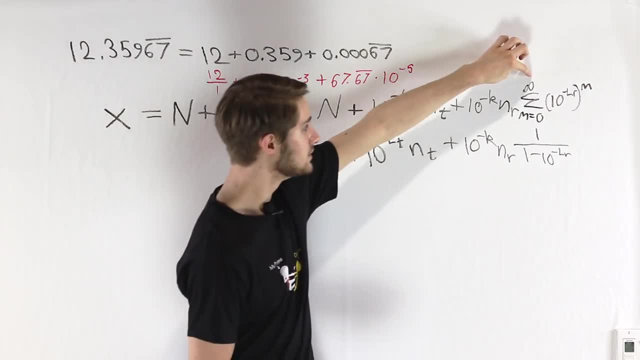 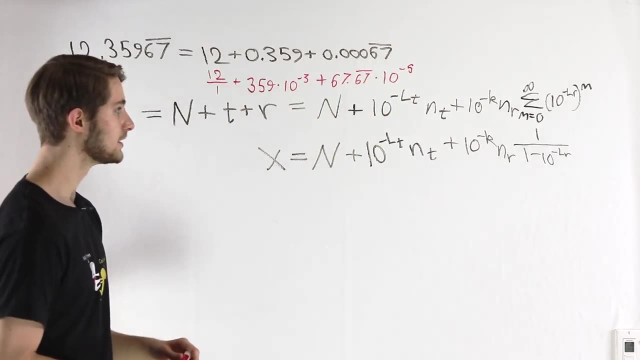 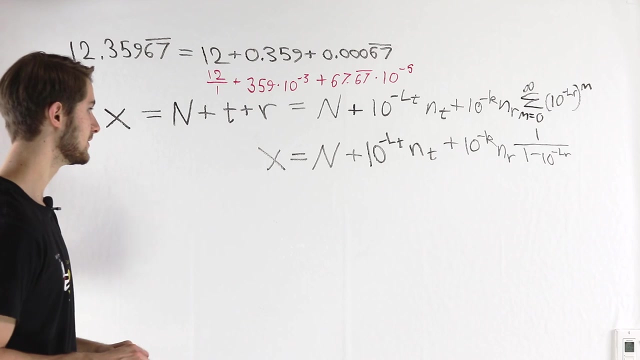 this part here which represents the evaluation of a geometric series where we add up every single instance of that repeating decimal sequence. Now, the important thing to notice here is that every part of this expression is a rational number: n, l sub t, n, sub t, k, n sub r and l sub r.